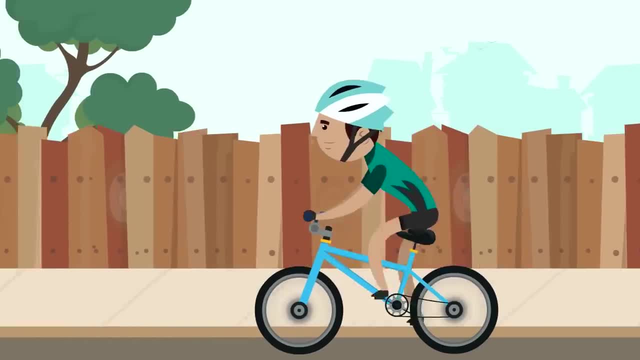 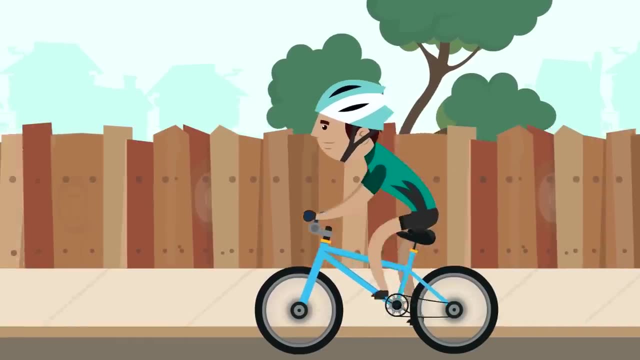 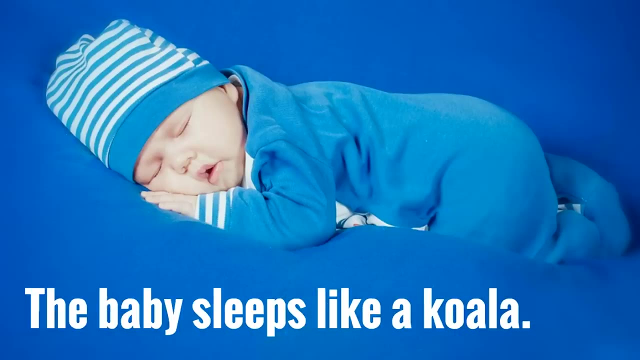 know what they are. Similes are actually a way of comparing two things. We compare things all of the time. Look at this comparison: The baby sleeps like a koala. In this sentence, we are comparing the baby to a koala. What's the comparison? That the baby sleeps like. 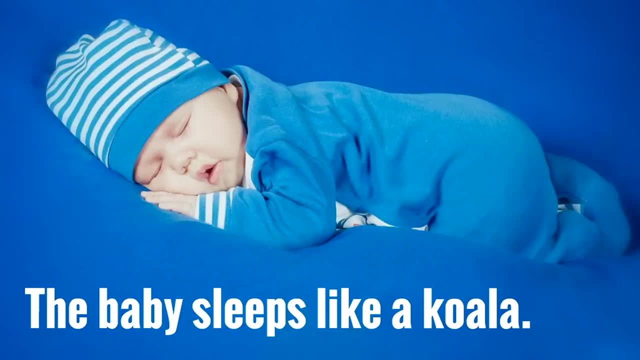 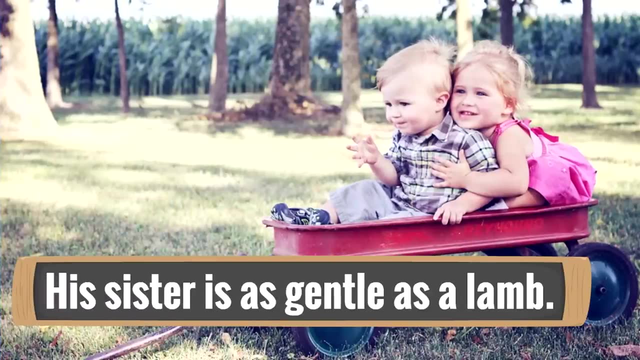 a koala. This is a comparison. Look at this comparison. His sister is as gentle as a lamb. His sister is as gentle as a lamb. The comparison is between his sister and the lamb, And the gentleness is what makes them similar. His sister is as gentle as a lamb. That's a comparison. 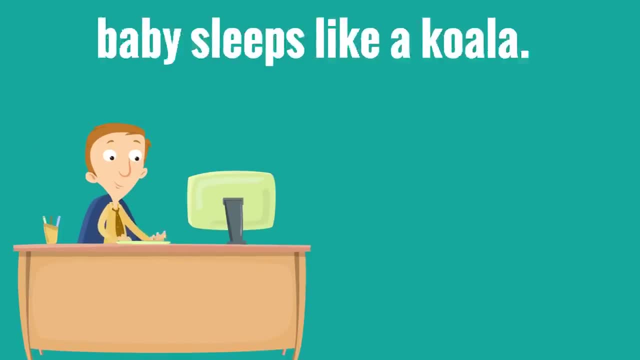 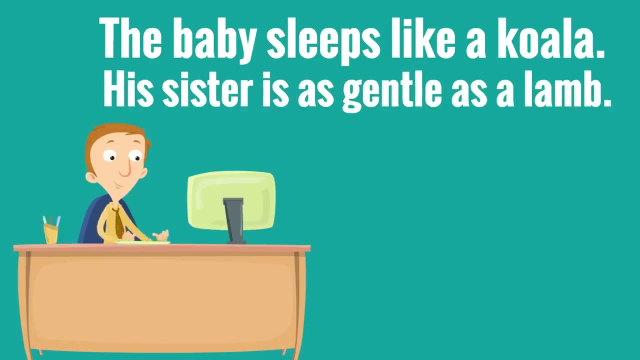 Let's look at both of our comparisons again. The baby sleeps like a koala And his sister is as gentle as a lamb. You want to know something interesting about these comparisons. These comparisons are similes. That's right. Both of these sentences are similes. 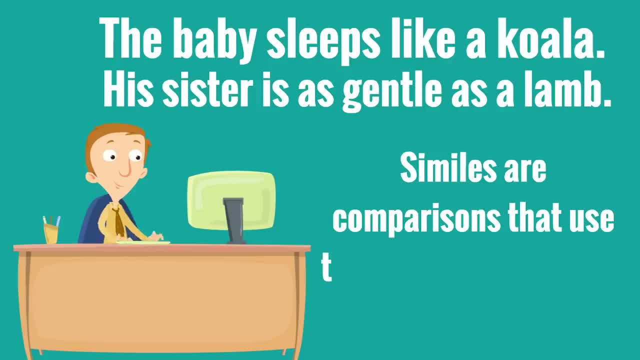 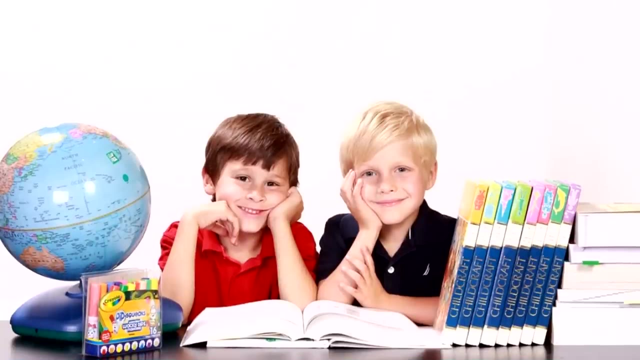 You see, similes are comparisons that use the words like or as. If there's a comparison that uses the words like or as, then you know that that comparison is a simile. Look at this sentence. Learning is as easy as pie. Wow, Learning is being compared to. 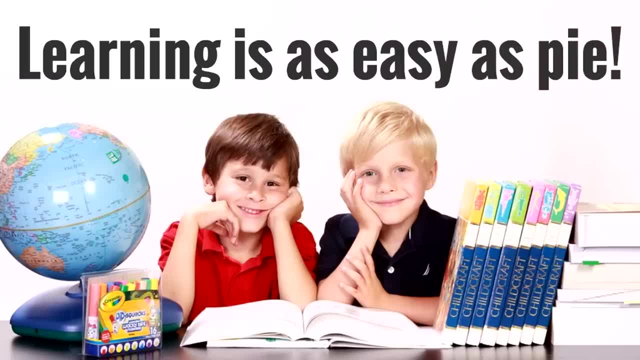 having pie Easy as pie is a very common simile. that means easy, Just like it's easy to eat pie. In this sentence, learning is as easy as pie. It's easy to learn. Learning is as easy as pie. CONSMISAL. 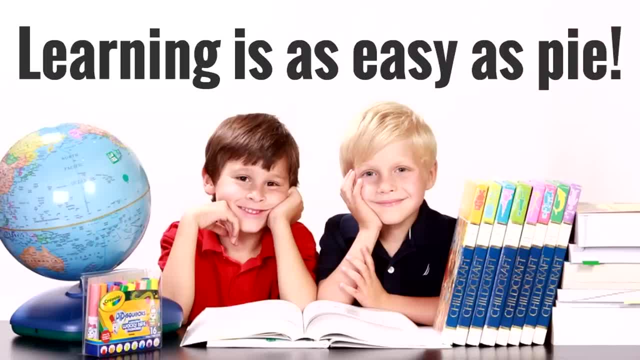 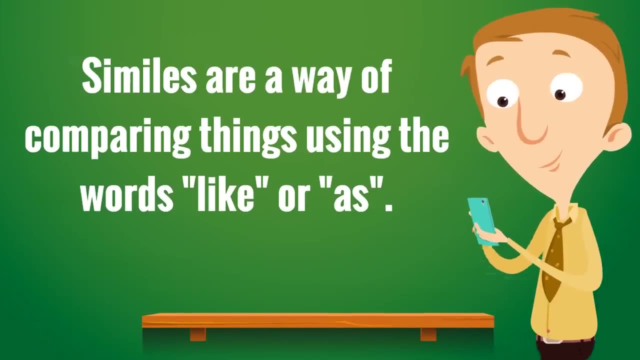 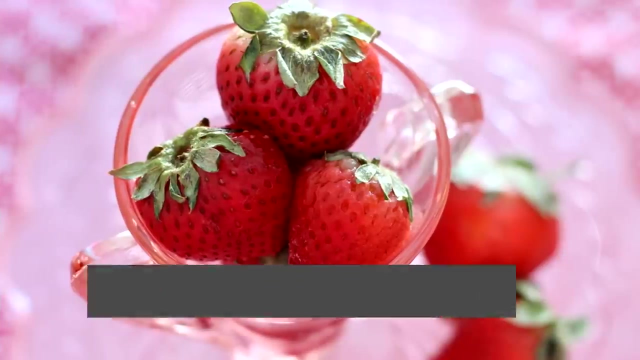 This is a simile because it is a comparison using the word as. Remember, similes are comparisons that use the words like or as. Similes are a way of comparing things using the words like or as. Look at this simile: The strawberries are red like roses.